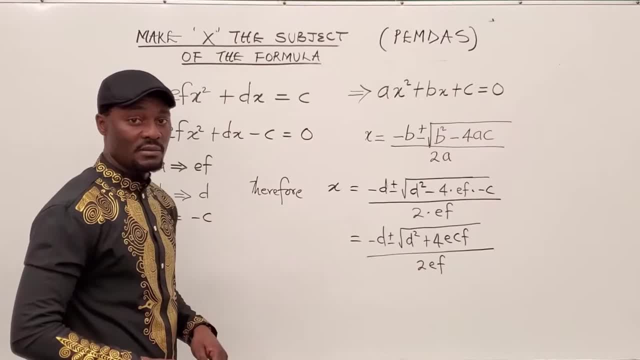 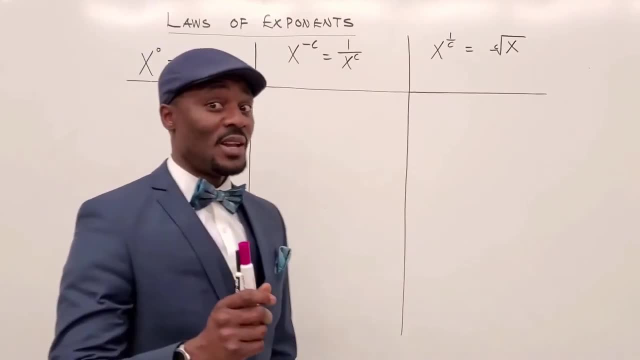 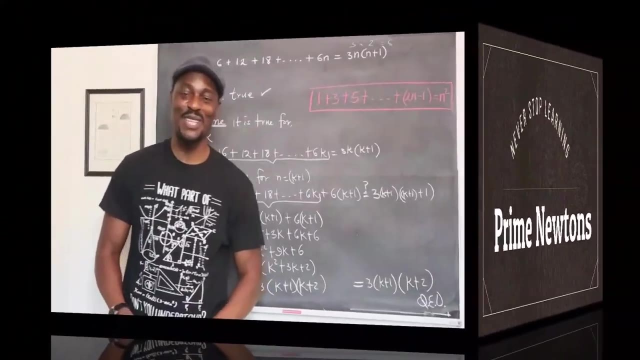 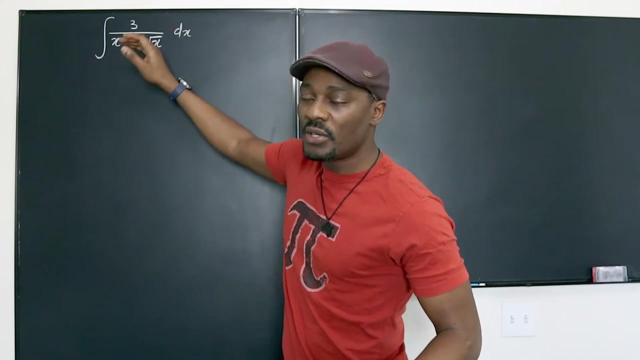 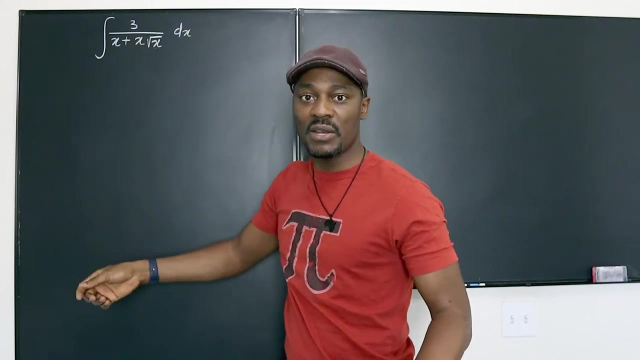 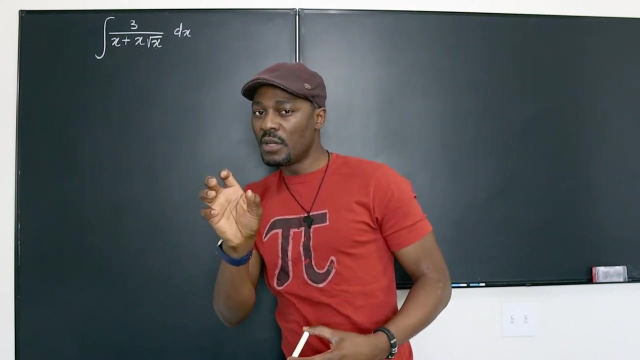 What you have is a rational function and you have x plus x, root x. Some people will just multiply these two together and get an expression, But I would rather view this as two terms, a polynomial or as look at this, because what I'm seeing right now is partial fractions. 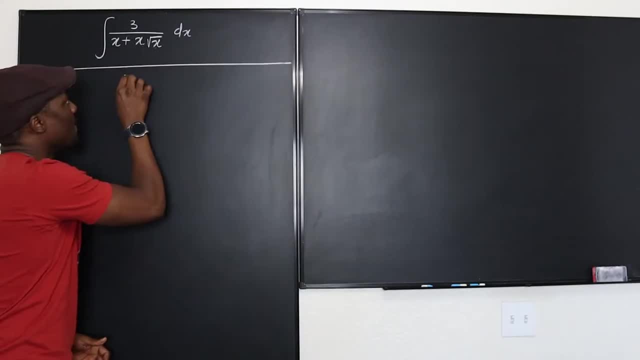 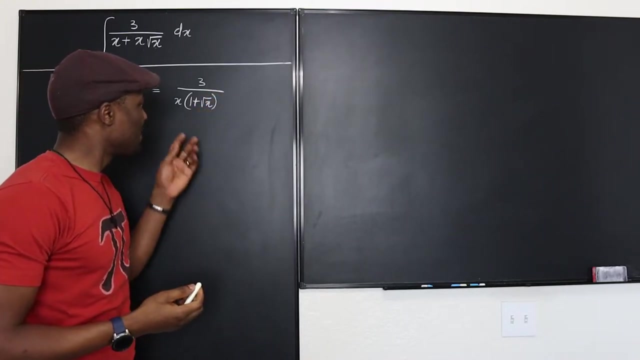 That's what I'm seeing. I don't know if you see it. 3 over x plus x root x. Well, I can factor this out. It will be 3.. 3 over x into 1 plus square root of x. So this looks like I've taken the least common multiple of two separate. 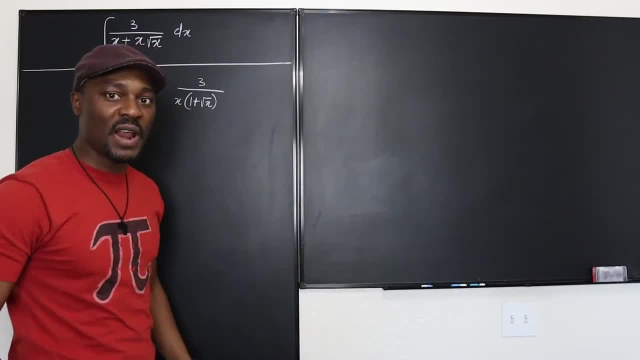 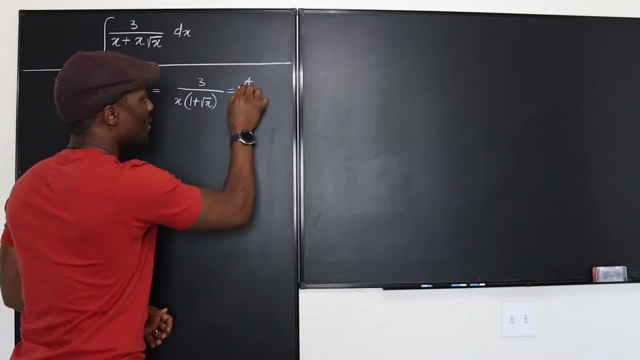 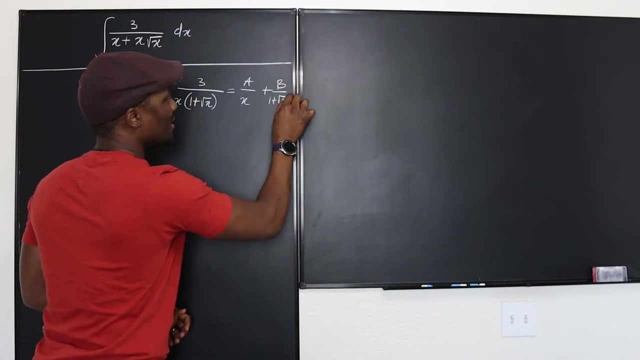 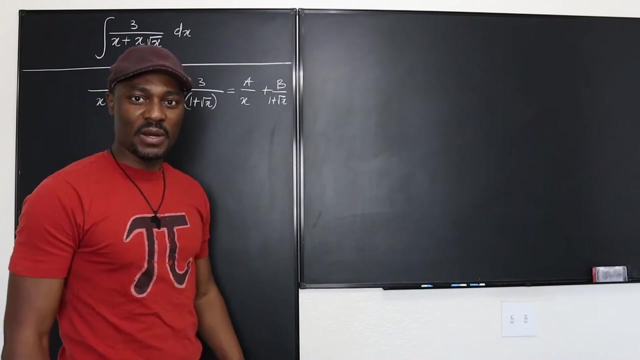 fractions. I want to break it down into those two separate fractions, using partial fractions, So I will rewrite this as a over x plus b over 1 plus square root of x. Well, this is not a polynomial function. It is not, So this is not going to work. 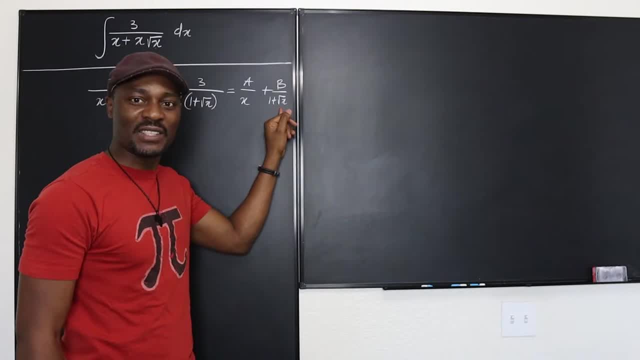 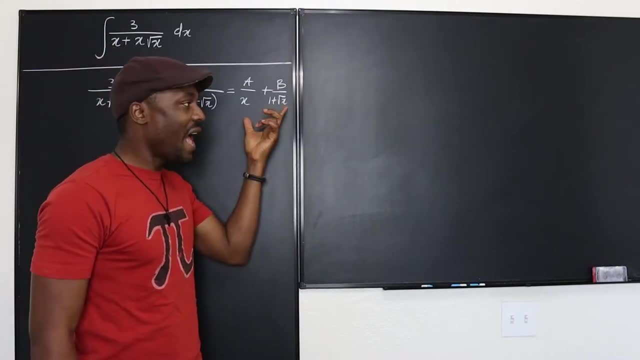 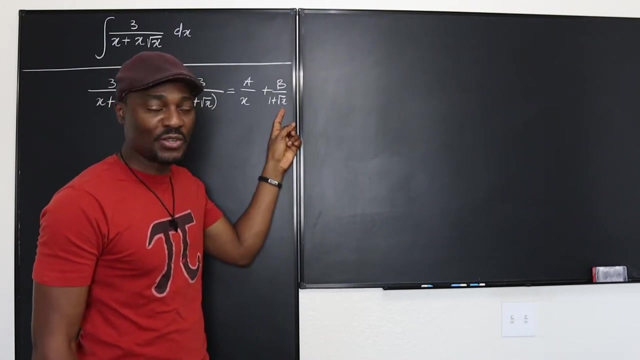 But can I change this so that it doesn't look like a square root stuff? Yes, I can actually change this so that by the time I get here, what I have can be a true polynomial denominator. Remember, you can't do partial fractions when you have irrational, because you don't know what this x is going to be. 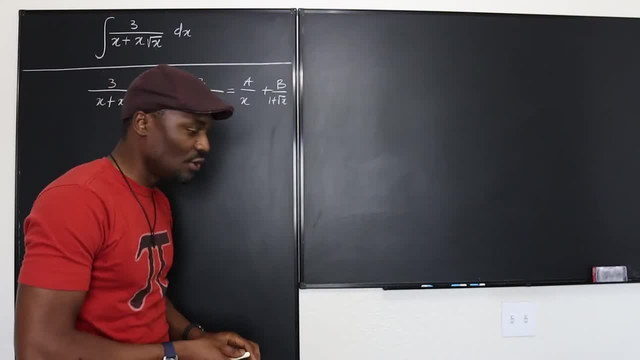 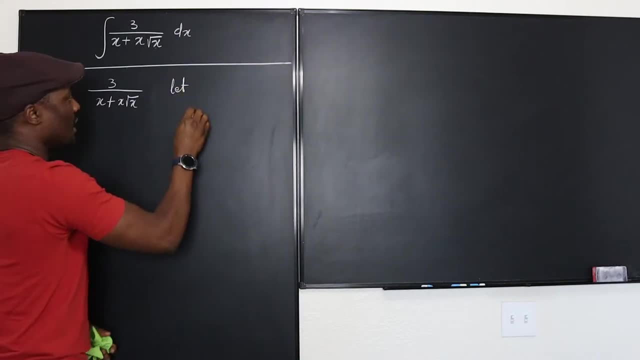 Okay, Irrational. So what you want to do is rewrite this function. Let's go back. I'm going to say: let y be equal to. let's not use y, let's use u. Let u be equal to the square root of x. 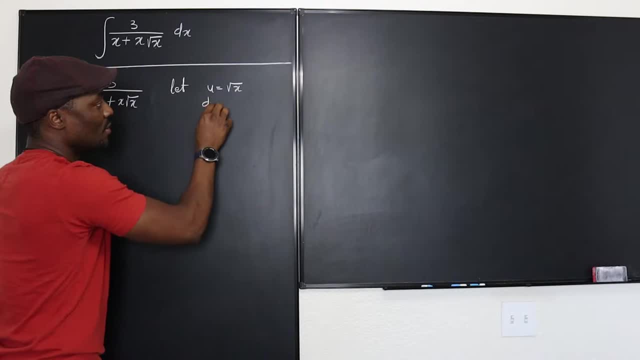 Okay, So that du will be equal to 1 half. We can do it that way. du will be equal to Let's, so that u squared- let's do it that way- u squared will be equal to x. Now you can differentiate both. 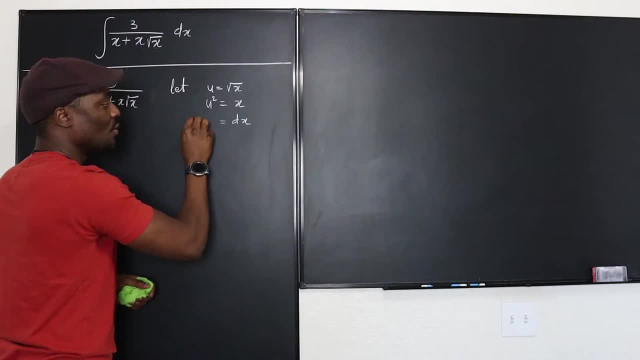 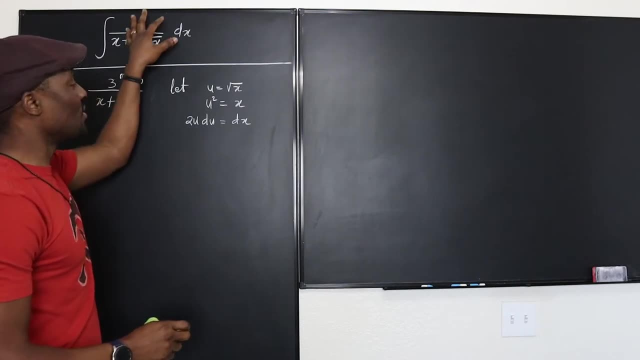 And then you have dx will be equal to 2u du. So now I can go here and replace this in this function so that this integral see what's going to now. the square root is gone. Okay, Now I can go back. 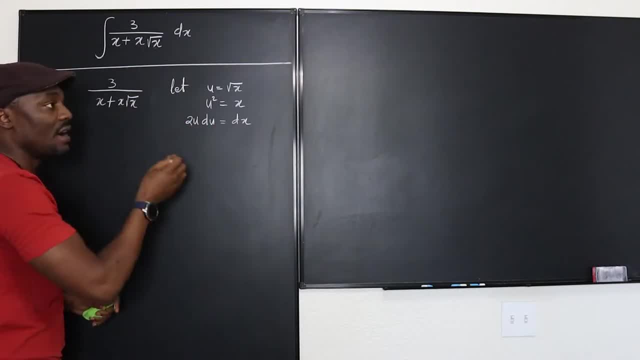 and replace dx with 2u du, And this, our integral, becomes the integral of 3 over what is x? x is u squared. I'm going to write u squared plus x times square root of x. That's going to be u squared times u. That's going to be u cubed. 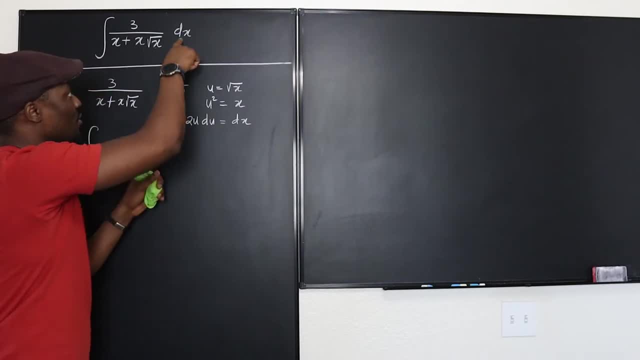 Brilliant. Huh, It's looking good. Now we need to replace dx, and dx is going to be 2u du Good. So what we have right now will be equal to 6u over. this is going to be u squared. 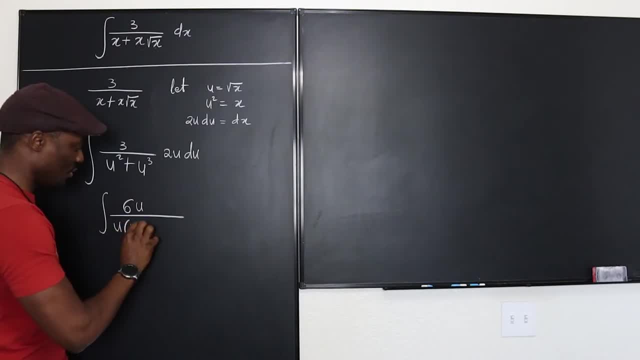 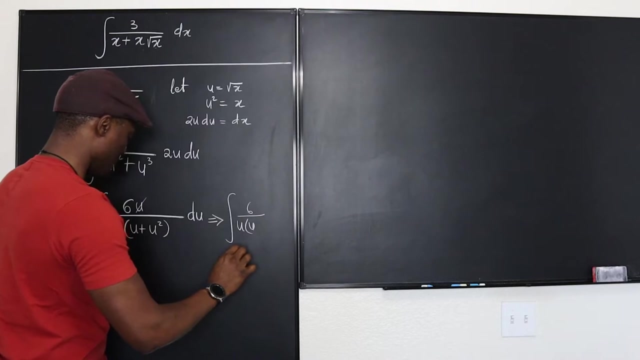 I'm going to say u into u plus u squared. Okay, That makes things easy: The u, this u can take this u out And what you have left will be the integral of 6.. I'm going to say u squared over u into u plus 1, or 1 plus u. so we follow the order 1u plus. 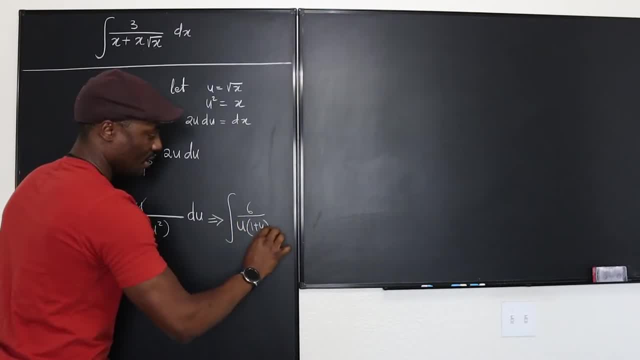 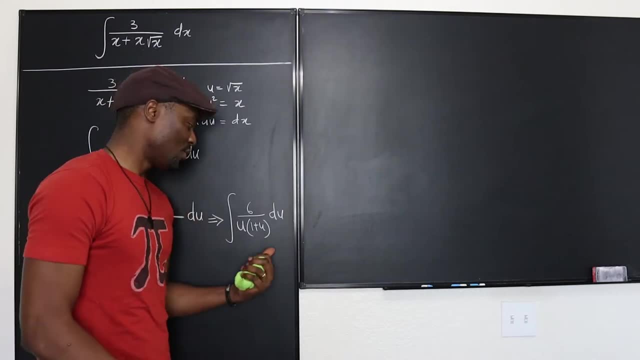 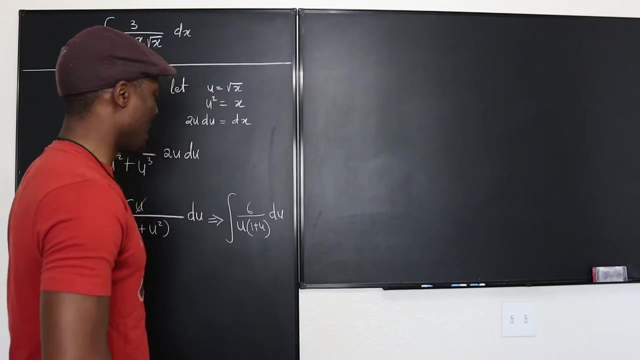 that's going to be u into 1 plus u. then you have du. Now this is easy for anybody to integrate. You just need to resolve this into partial fractions, because that's the only way out and we'll be good. Okay, So let's do that. Let's resolve this into partial fractions. 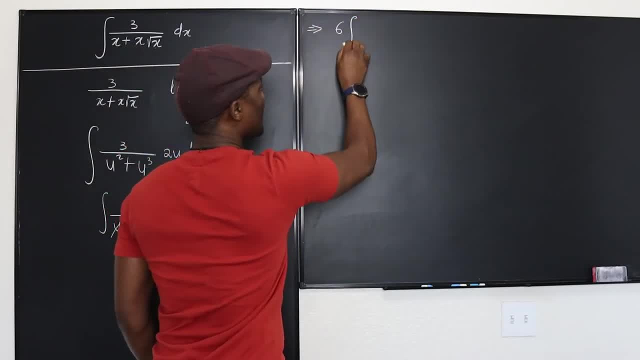 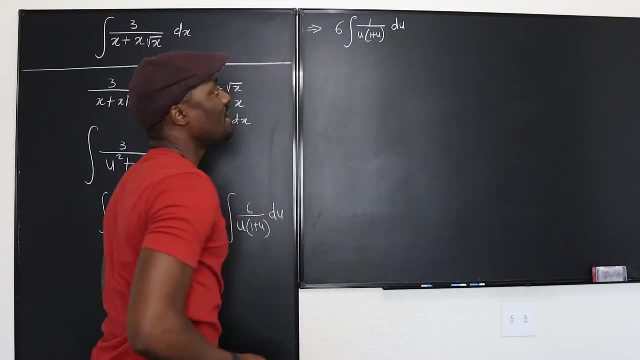 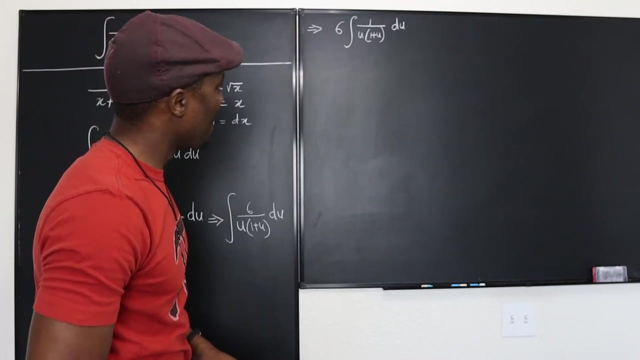 So this implies 6 integral of 1 over u into 1 plus u du. So resolving this into partial fractions. let's do some little tiny paperwork on the side. I'm going to do it here. I'm going to erase it over time, but if you don't understand partial fractions, 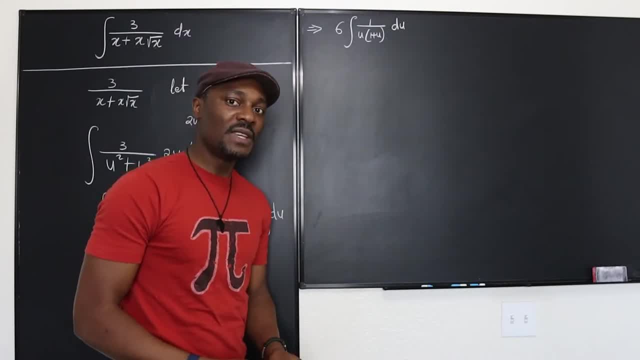 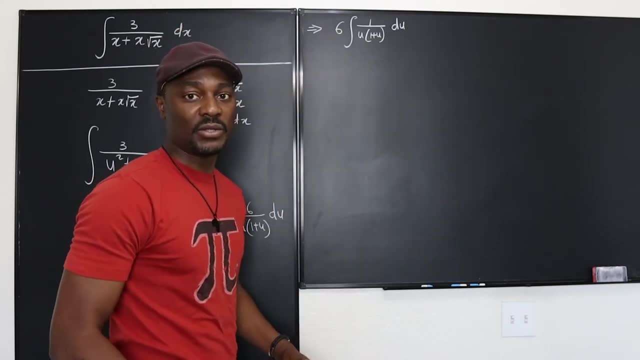 um, I think you should watch my next video or one of my previous videos. I didn't really do much, but I can do a comprehensive video on all of the techniques in partial fraction. Okay so, and that's going to come next. 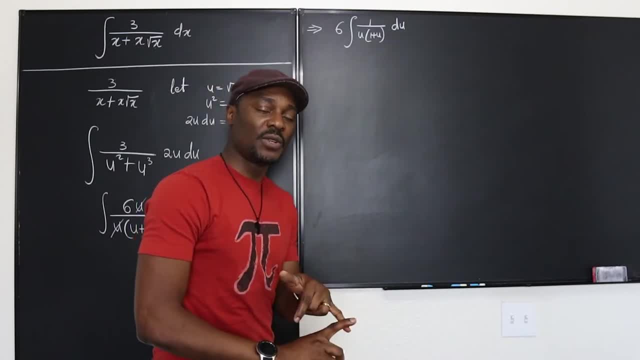 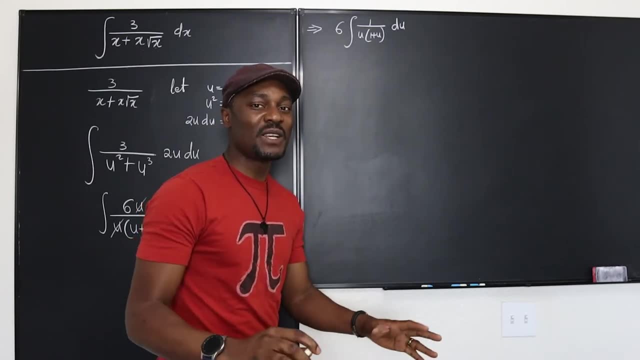 So what we have. so if you're a pre-calc, pre-calcular student or you're a Calc 2 student, you must have partial fractions taken care of, because they are very relevant to what you're doing. So at this point we're going to resolve 1 over u. 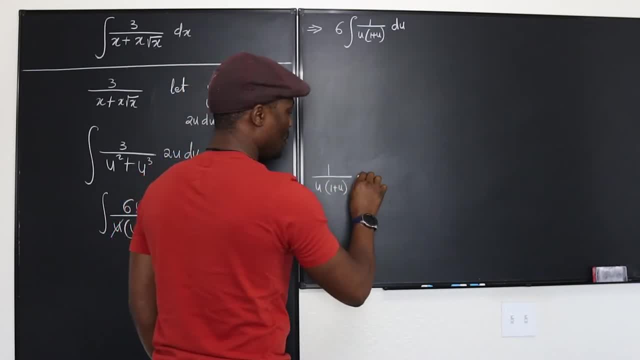 into 1 plus u, okay, into partial fractions. So it means this is: these are two terms multiplying each other. That's a over u, okay, plus b over 1 plus u- okay. Since this is the least common multiple, we're gonna multiply everything by u into 1 plus u. 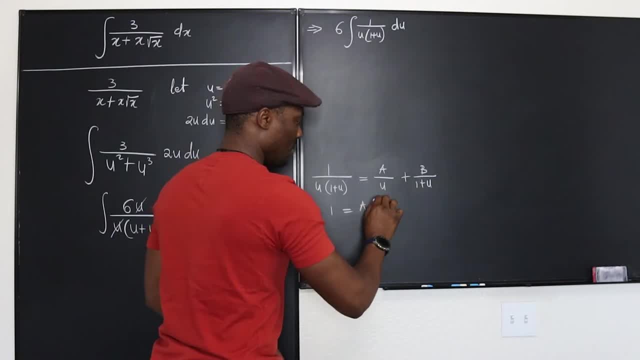 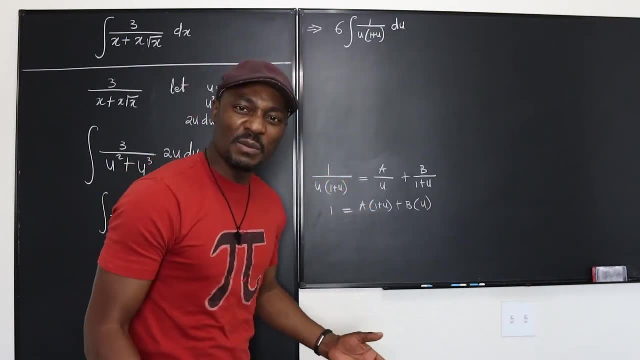 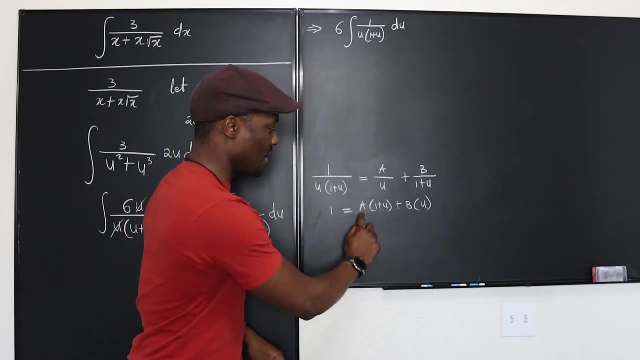 You'll end up with 1 equals a multiplying 1 plus u and plus b multiplying 2.. u Okay, let's do some very smart things. What if, when u is 0, you see, when u is 0, this is going to be 0, and what you have is going to be a times 1, and this is going to? 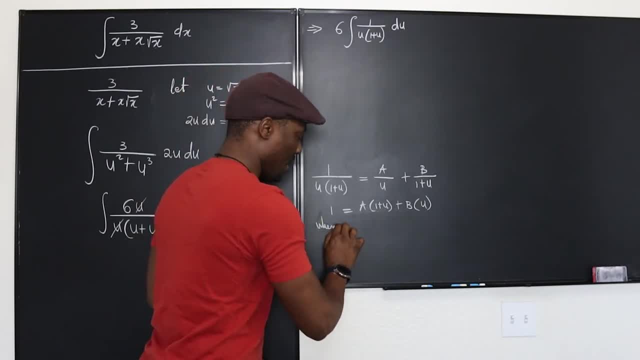 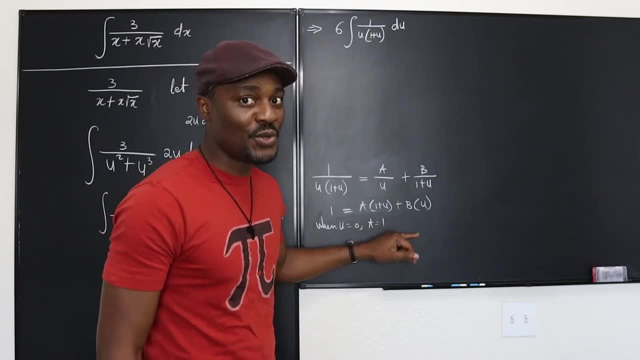 be just 1.. a is going to be 1.. Okay, when u equals 0,, a will be 1.. At least we know what a is. Remember: a is constant. It doesn't matter what u is. but we've been able to smartly. 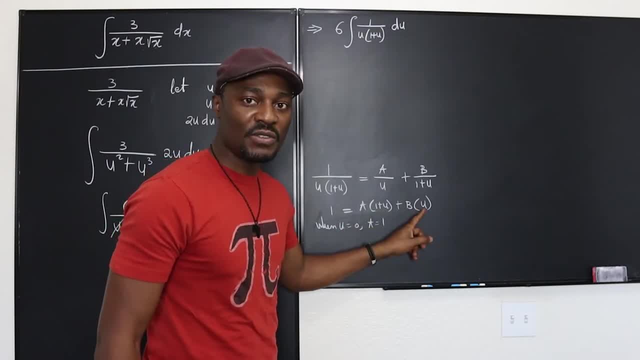 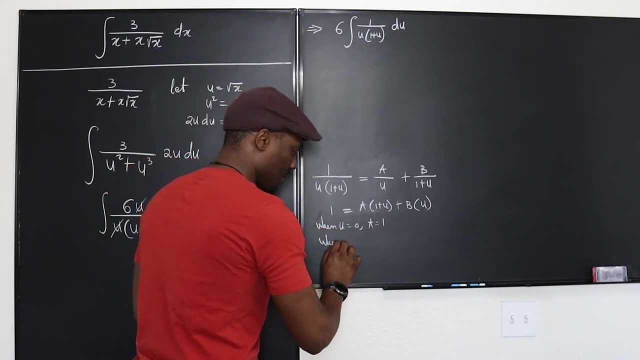 find what a will be by just putting u equals 0.. Now the smart thing to do to make this 0 is to make u negative 1, and if you do that and you can also say: when u equals negative 1,, this is going to be 0, and this is going to be negative b. Negative b equals 1, which. 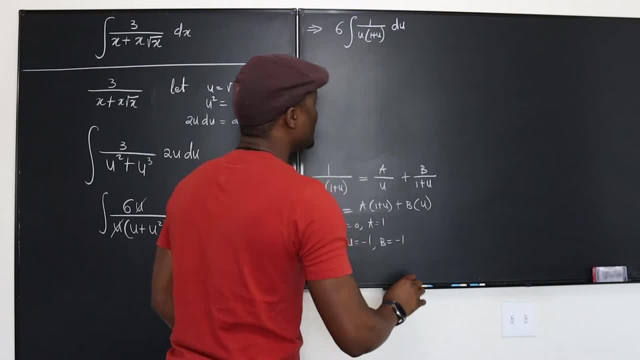 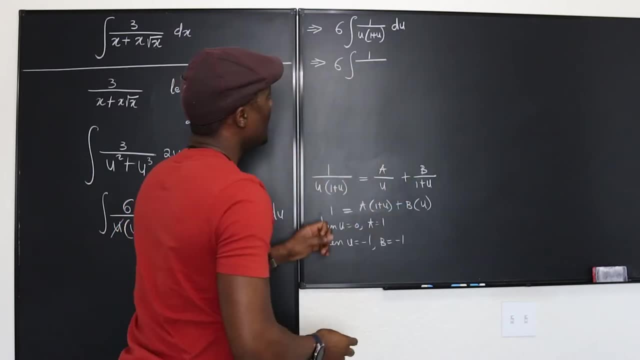 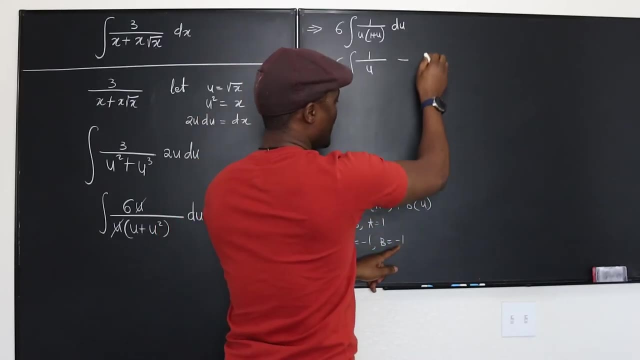 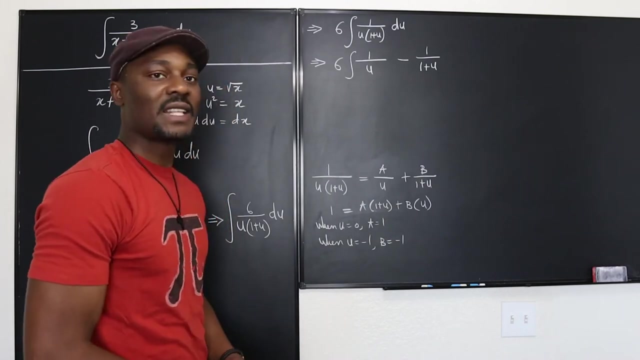 means b is negative 1, so b equals negative 1.. So we can actually resolve this into 6 integral of 1 over. you see it's a over u, That's 1 over u minus, because this is negative 1, minus 1 over, 1 plus u. That's it du. 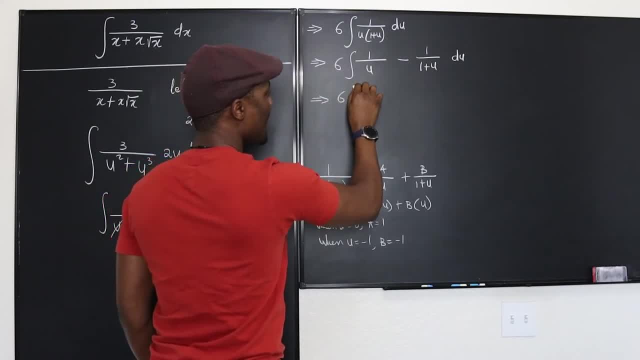 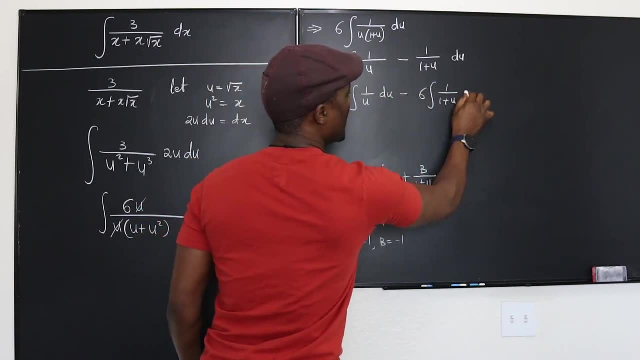 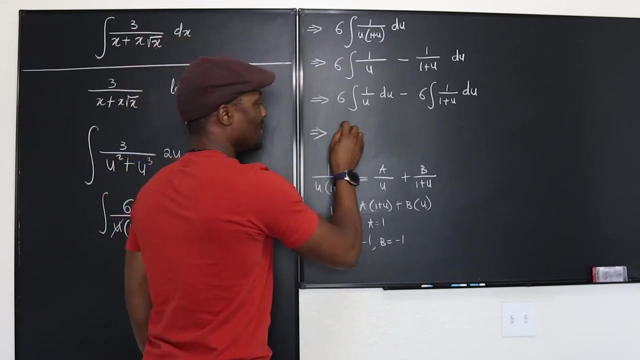 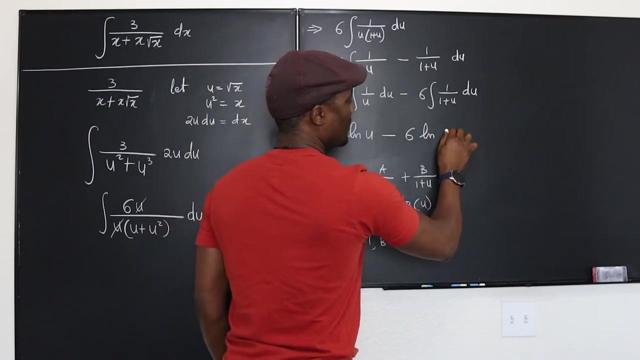 Let's integrate. This is 6 integral of 1 over u du minus 6 integral of 1 over 1 plus u du. Ladies and gentlemen, what we get is 6 ln u minus 6 ln. 1 plus u absolute value. Let's use the absolute. 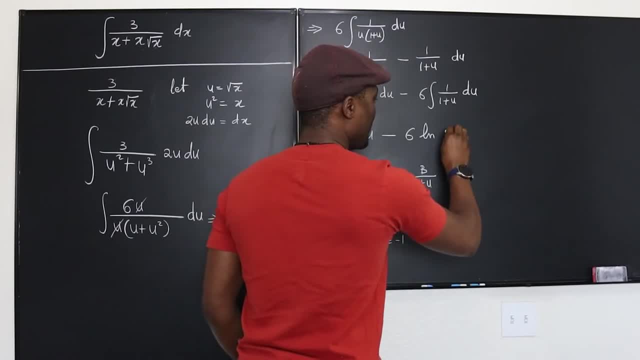 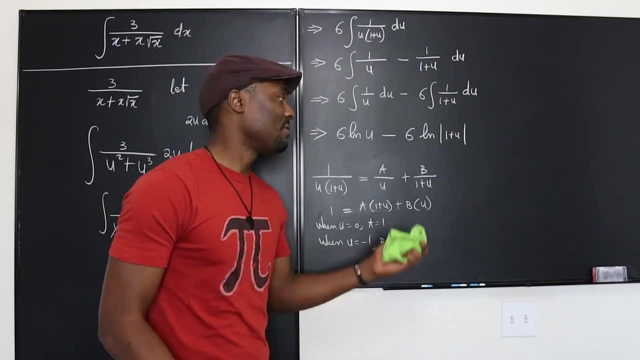 value side. okay, I like doing that. You don't lose any points for putting the absolute value. Well, if you figure out you don't need to put it, then you can change it, but I just leave it. Nobody puts it. 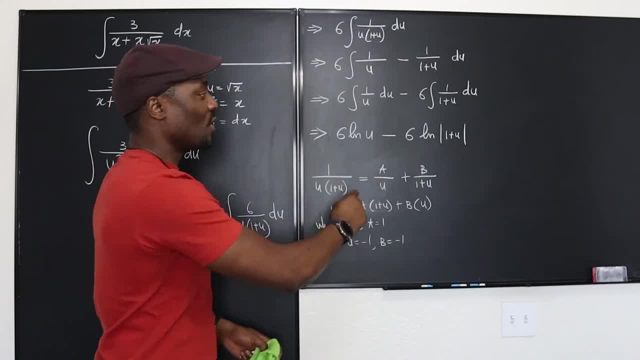 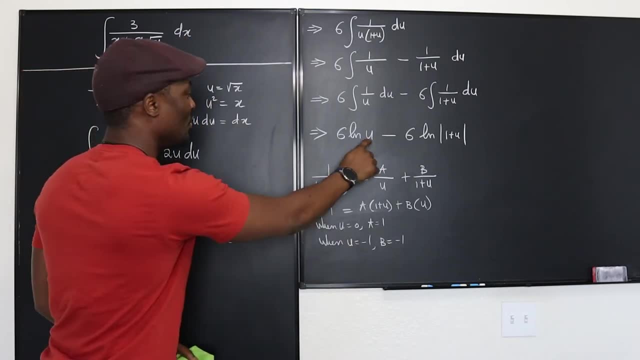 Subtitles by the Amaraorg community punishes you for that, Okay, well, this question was not about u, not about u, it's about x. So we have to go back and replace u. Remember, u is the square root of x. So we're going. 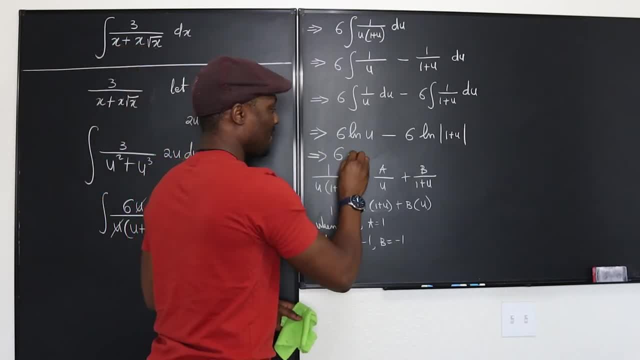 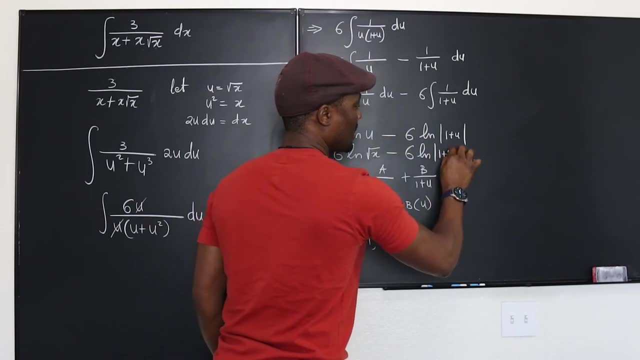 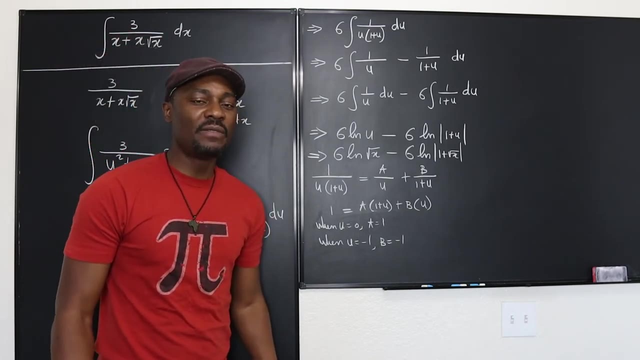 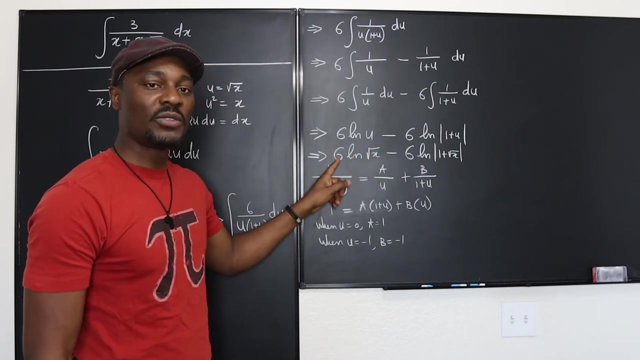 to rewrite this. okay, This is going to be 6 ln root x minus 6 ln 1 plus the square root of x. Okay, and that should be our final answer. However, you know you can actually write this as x to the 1 half. Take the 1 half, use it to multiply this. 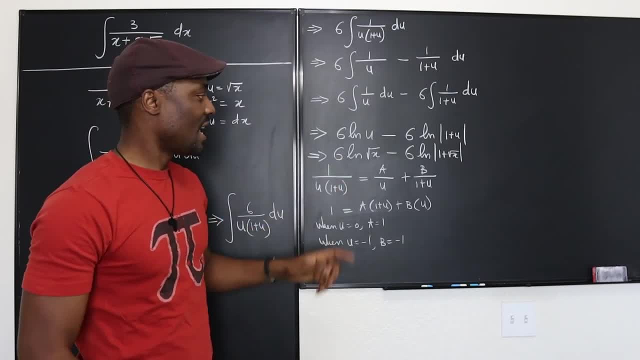 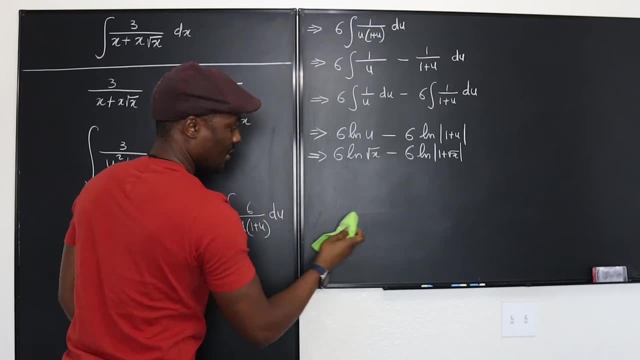 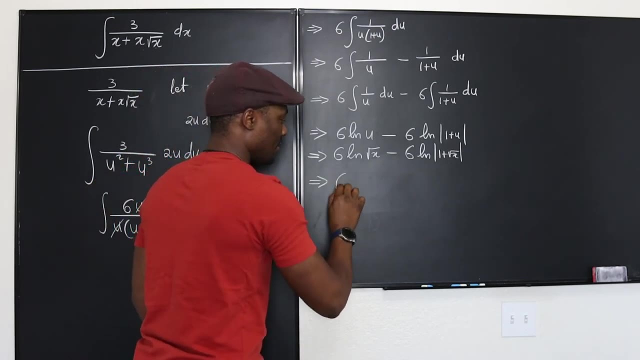 That's going to be 1 half of 6, and you can actually change this, So I'm going to take this off. Let's do it. So this is going to be 6 ln x to the 1 over 2.. 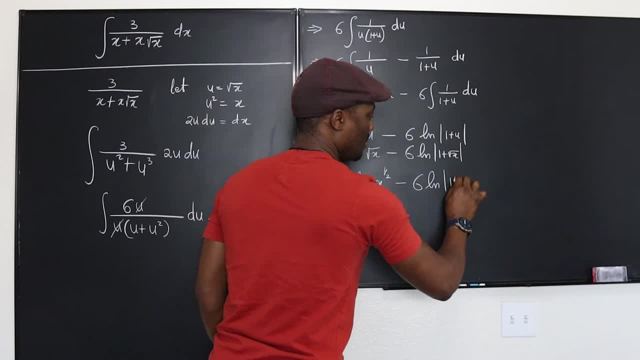 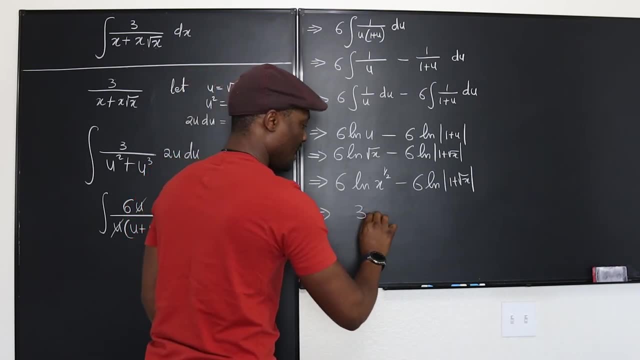 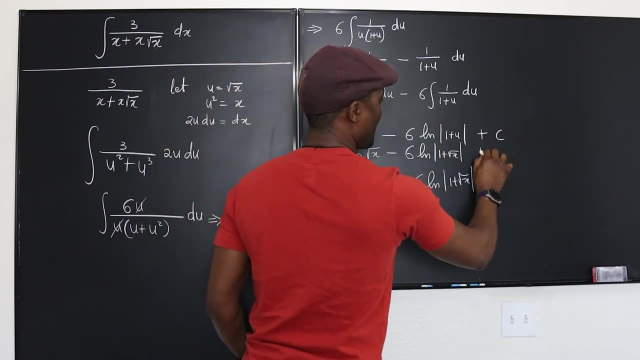 Minus 6 ln 1 plus the square root of x. So this 1 half goes here and divide 6.. That gives you 3 ln x. You don't have to do this. This is good enough as an answer. Plus c: I forgot Plus c. Don't forget that. 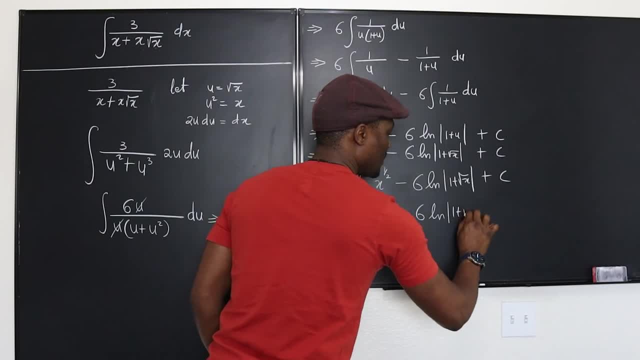 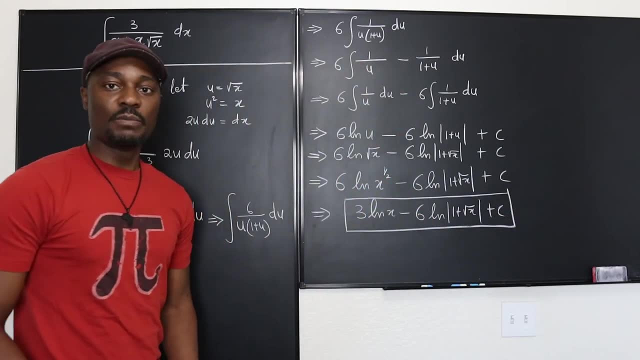 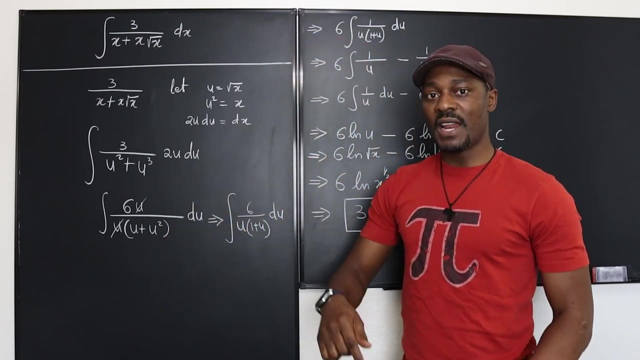 6 ln. 1 plus the square root of x Plus c. That's what you're supposed to get. I hope you learned something, okay? If you did leave a nice comment in the comment section, Make sure you're subscribed. if you're not, Share this video. Talk to your friends about it, okay. 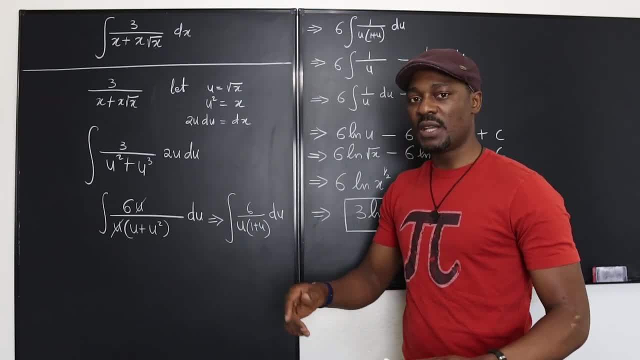 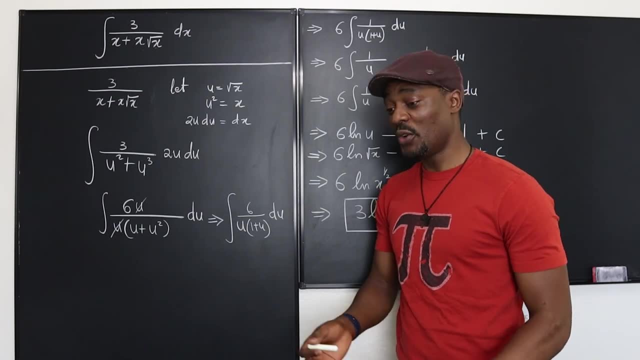 If you have any specific question you'd like me to help with, just send me an email. It's just the name of this channel at gmailcom- primemutants at gmailcom- And I'll get it and I'll make a video for it. Or leave the question in the comment section. I'll find it. 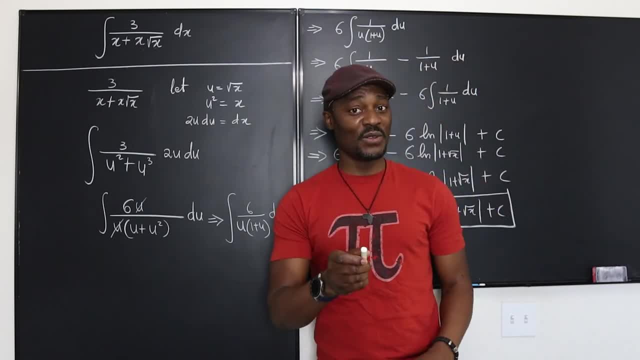 Take care of yourselves. See you in the next video. Don't stop learning, because those who stop learning have stopped living. Bye-bye.